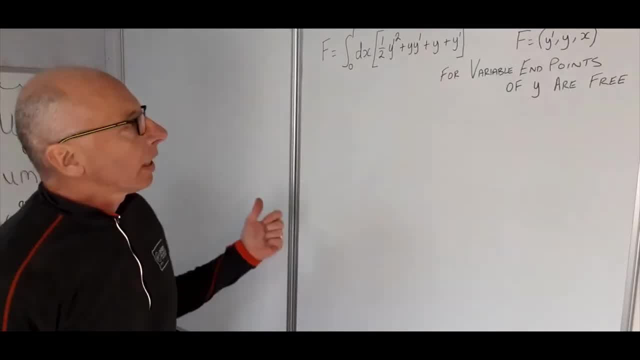 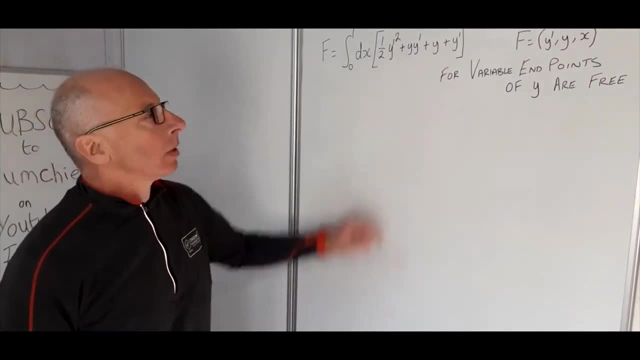 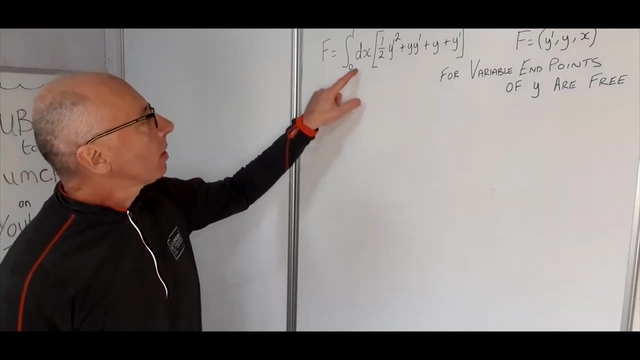 Okay, so we've got a calculus of variations problem here and this particular question is a variable endpoint problem. Now the endpoints of y are three. we don't know what they are, but we're given that our x values are from zero and one, That's our range of the integral. 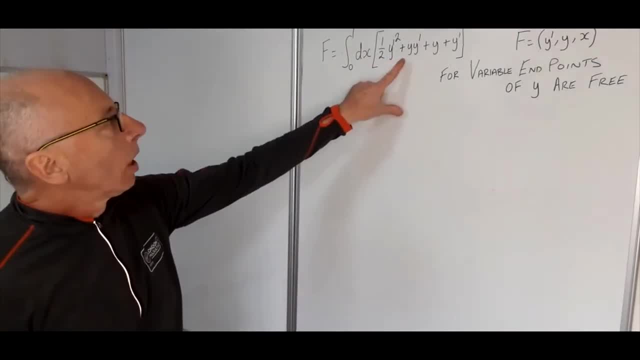 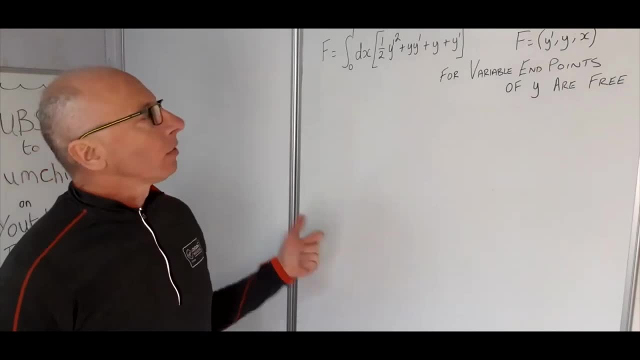 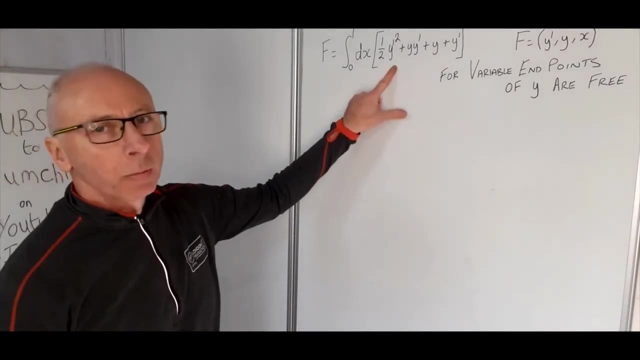 here. So we've got our y primes and our y's inside the functional. So how we can find the value of y of x from that is what we're really interested in. So the Gatto differential here could take quite a bit of time, could be quite complicated. The easiest and the 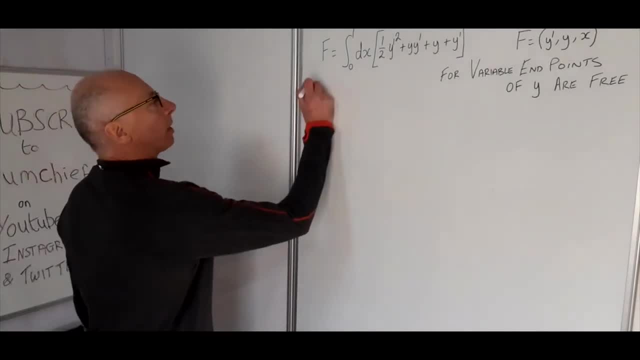 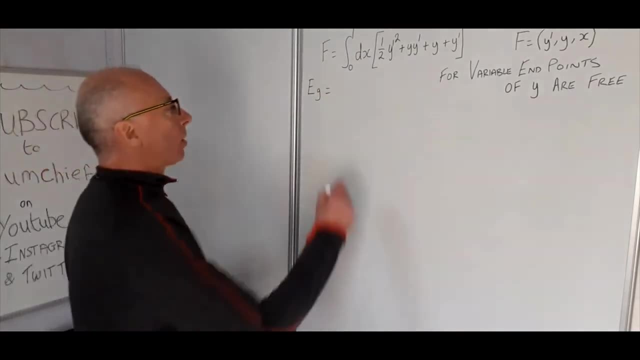 quickest route of that is going to be the Houlis-Lagrange equation. So that is written as so: partial derivative of this functional with a derivative of this functional, with a derivative of this functional, with a derivative of this functional with regards to y. And then we subtract from that the derivative with regards. 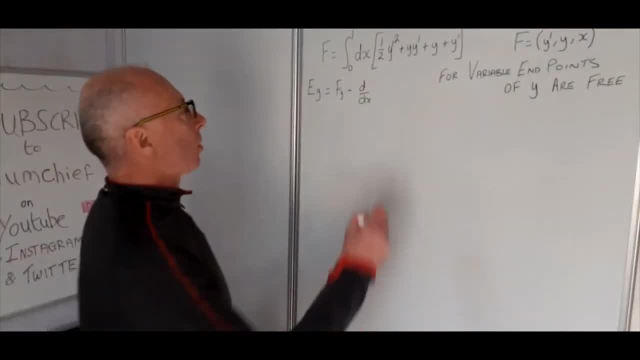 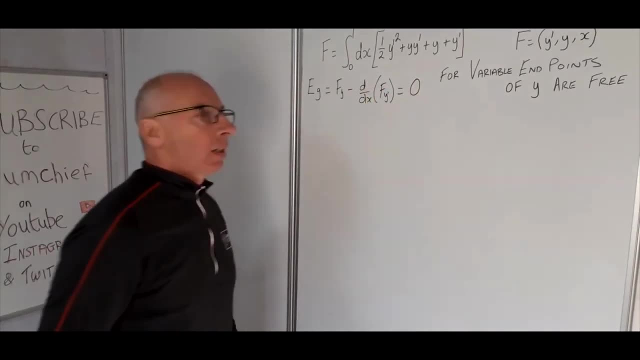 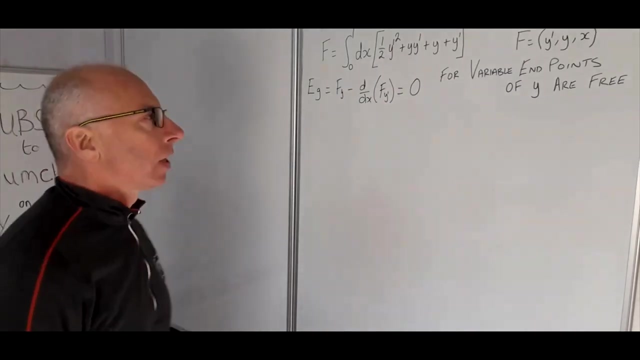 to x of the partial derivative of the functional with regards to y prime, And then we set that to zero, Because when the partial derivative and the derivative of the whole thing is set to zero, that's what we're interested in: to find these variable endpoints. 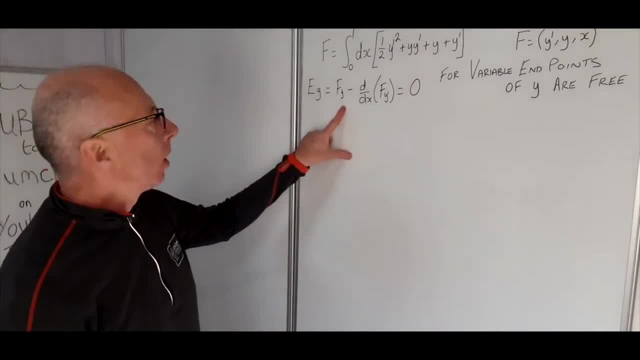 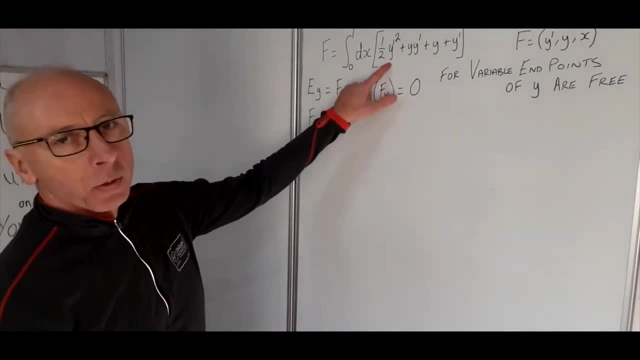 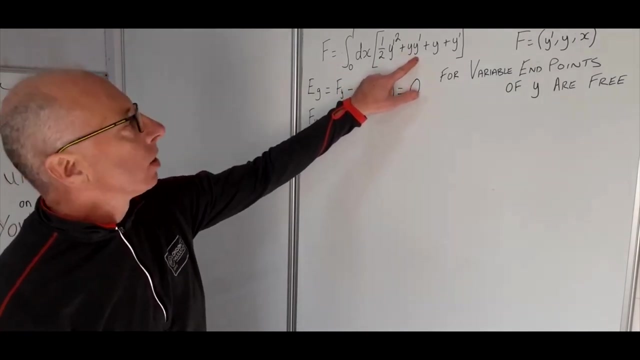 Okay, so first of all, let's find the partial with regards to y, So partial with regards to y, So the y prime squared. that's not part of this, so that's disappeared. So we've got a y and a y prime, So the y prime acts as: 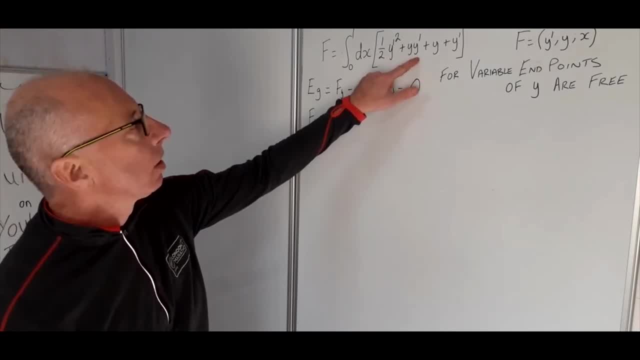 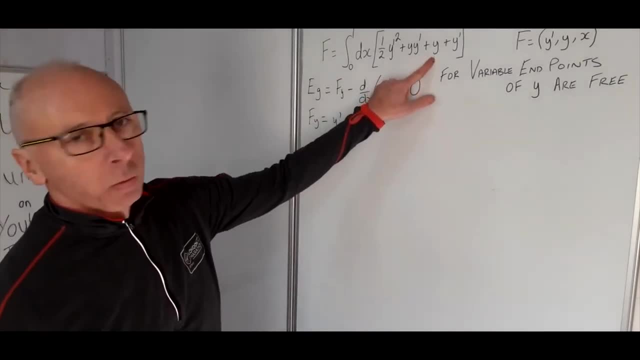 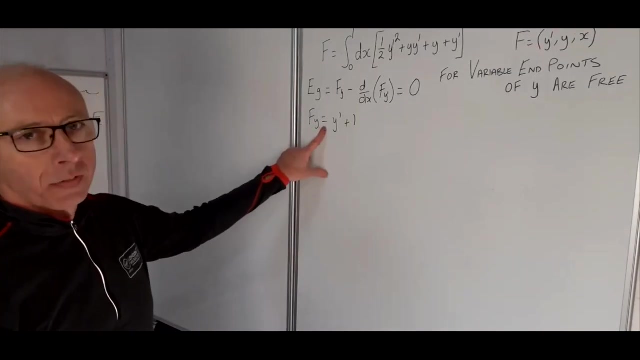 a constant multiple. So if we take the derivative of this, we're just going to be left with the y prime. Take the partial. with regards to y, we end up with a one And the y prime here we can disregard. So that's our first part of the Euler Lagrange. Now the second part, we'll take the partial. 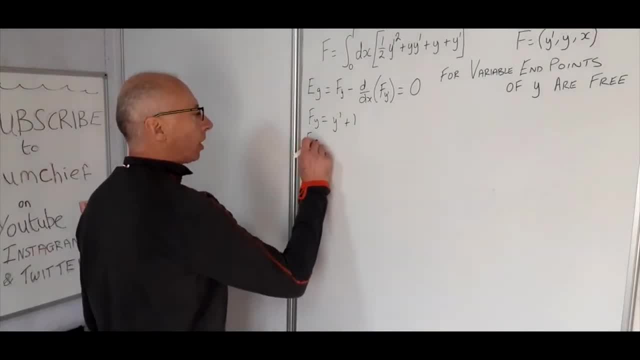 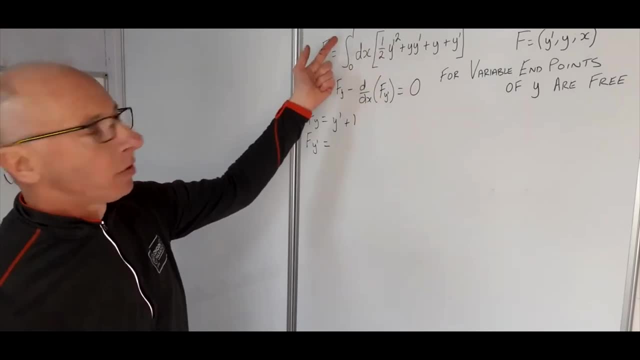 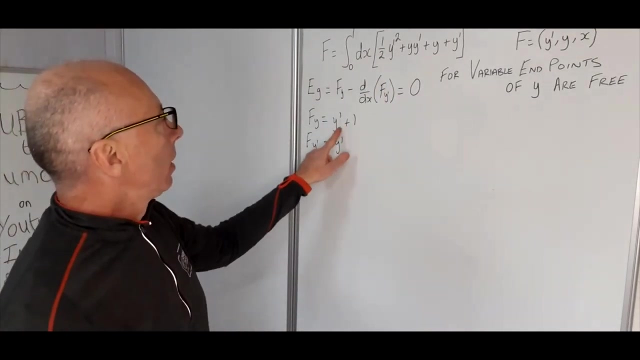 with regards to y prime. Okay, partial of this, bring the two out front. So then, two over two gives us a one, And the y prime squared just becomes y prime. So, as we did in this one, the y prime is what we're trying to find the partial of. So the y is now the constant. 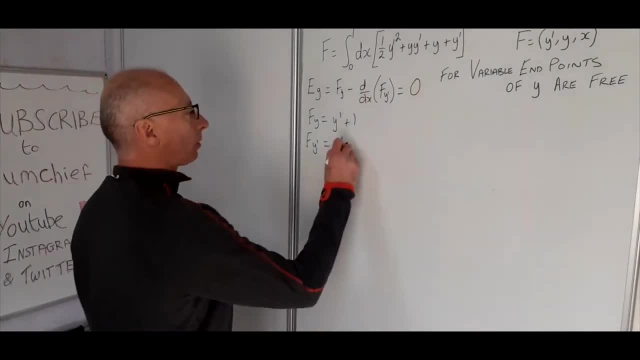 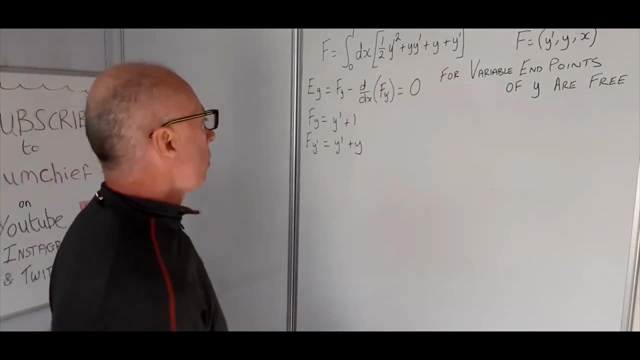 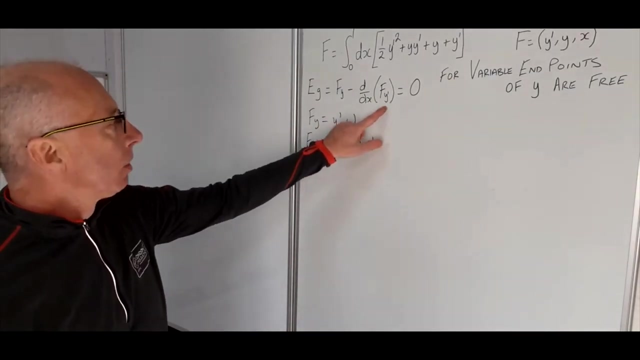 multiple. So that's just going to leave us with the y. This we can disregard. we're only interested in y prime, And then this will then leave us with a one. Okay, so now we need to take the total derivative with regards to this y prime. So now we take d dx of y. 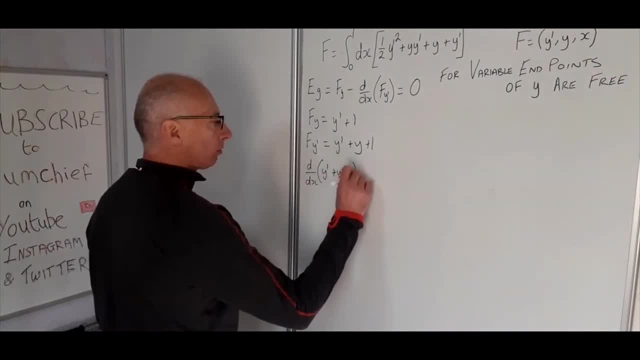 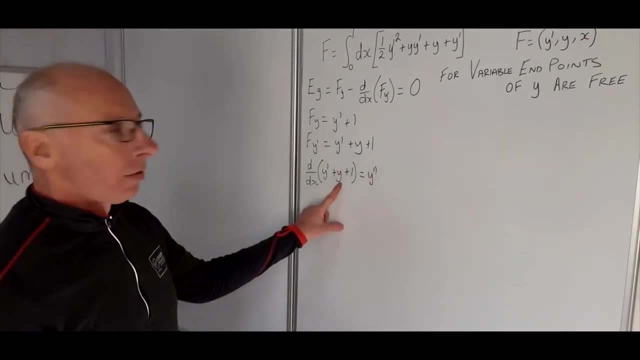 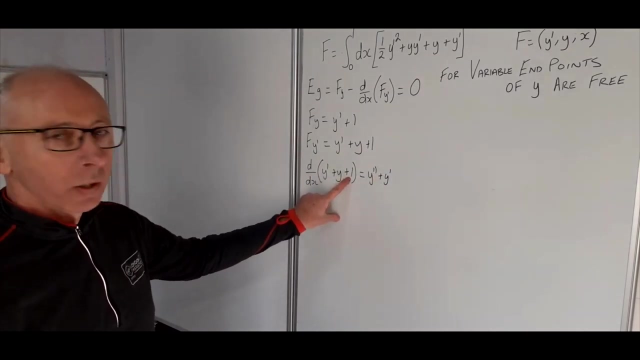 prime plus y plus one. So the derivative of y prime is 1 plus y plus one. So we're left with a one. This is going prime is just going to leave us with y double prime. Derivative of y is again y with the derivative, that's y prime, and the derivative of 1 is just going to. 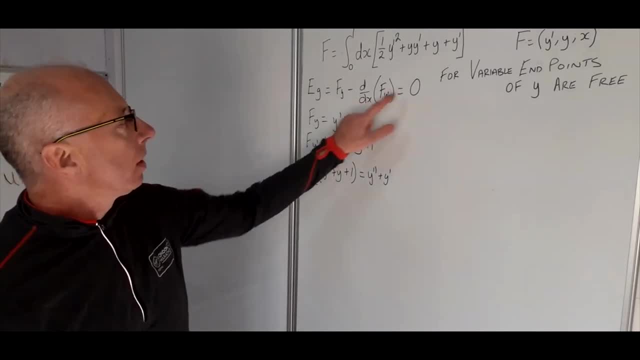 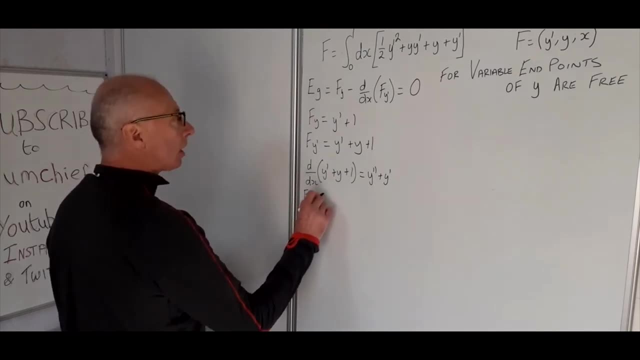 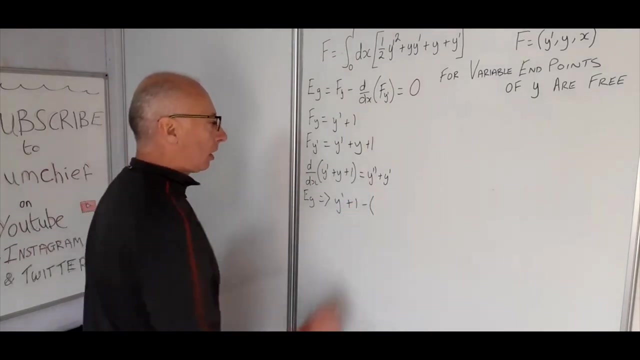 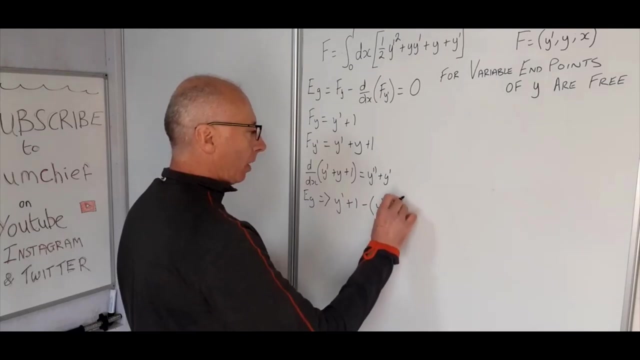 disappear. So now we're ready to write this in this form. So f of y. so I'll just write here the Lagrange equation just for that: f of y is y prime plus 1, and then subtract what we have here. So then we're left with y double prime plus y prime and set. 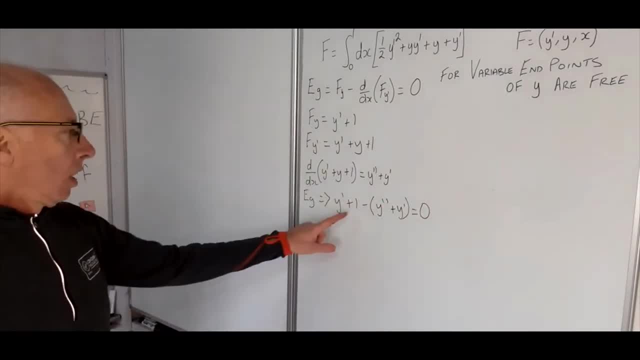 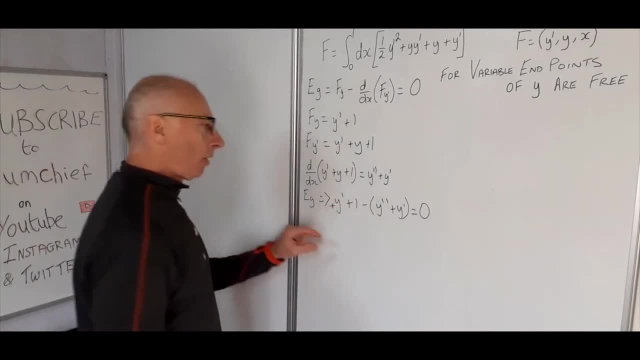 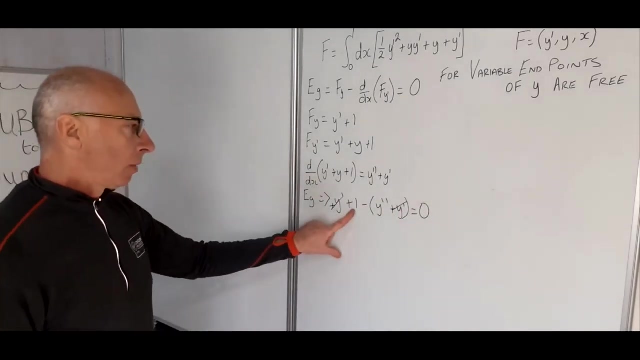 that to zero. Okay, so some simplification we can do. here We've got a y prime and a y prime here. This one is positive. Distribute the negative, this one's a negative, So these two will cancel out, and then we're left with 1 minus y. 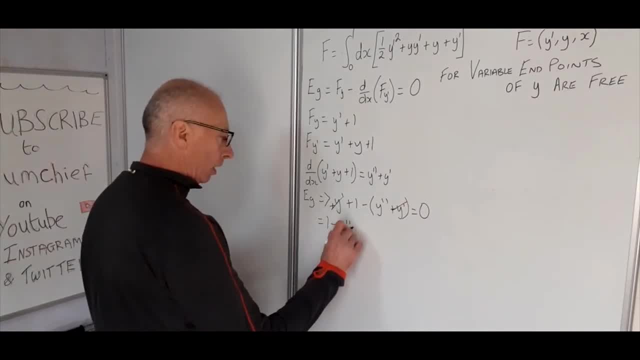 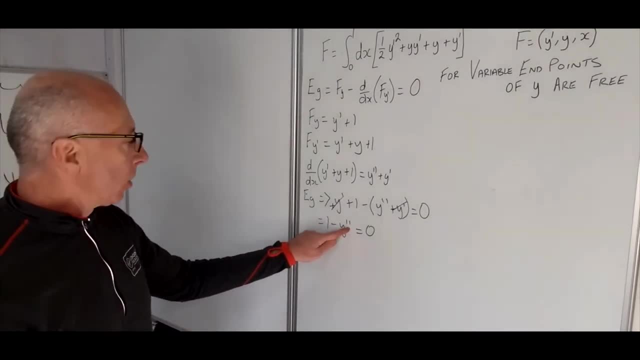 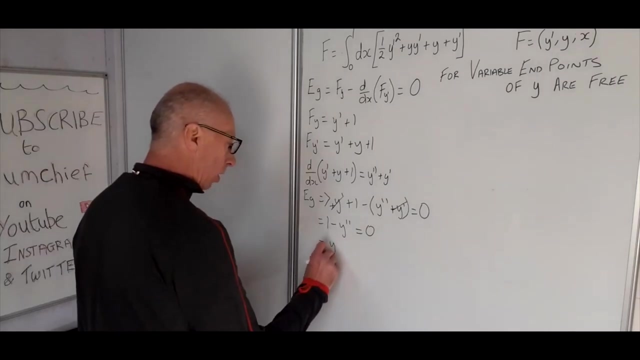 double prime Equals 0.. I always like to bring my highest order of my partials out to the front. So if I do that and multiply everything through by minus 1, I'm going to get y double prime minus 1 equals 0. So that's our Euler-Lagrange equation. So 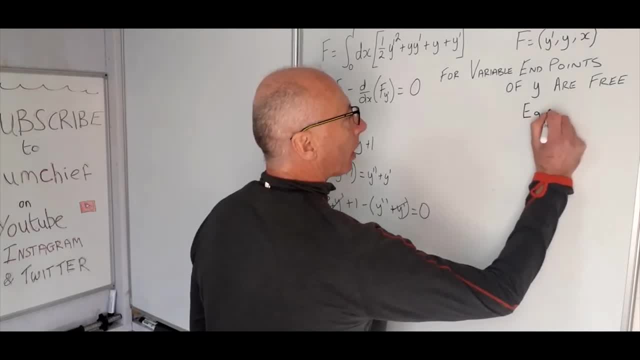 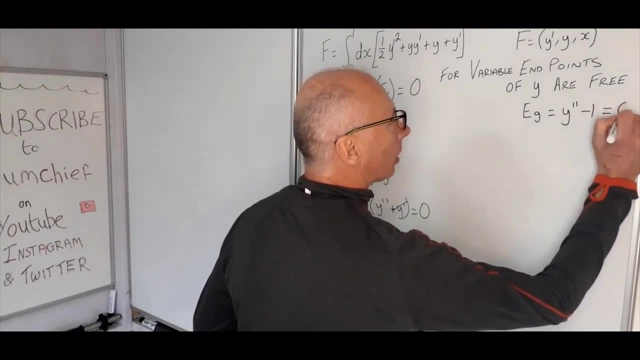 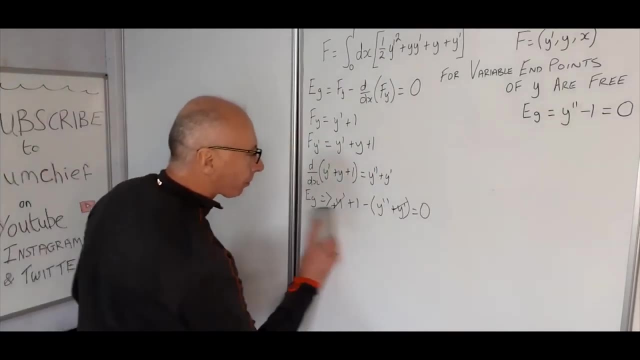 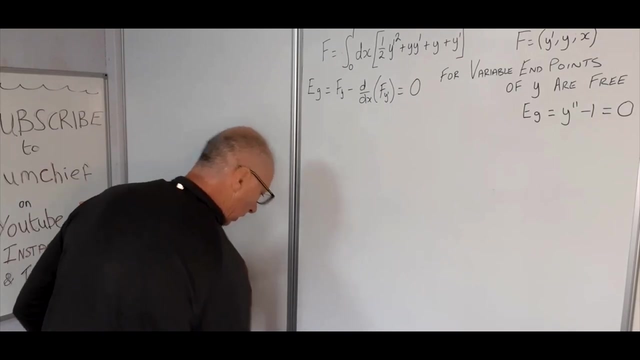 I'm going to put that up here. So my Euler-Lagrange equation is: y double prime minus 1 equals 0.. Okay, so I'm going to take this off the board, pause the video, and you can keep that if you want to write that down. Okay, so now. 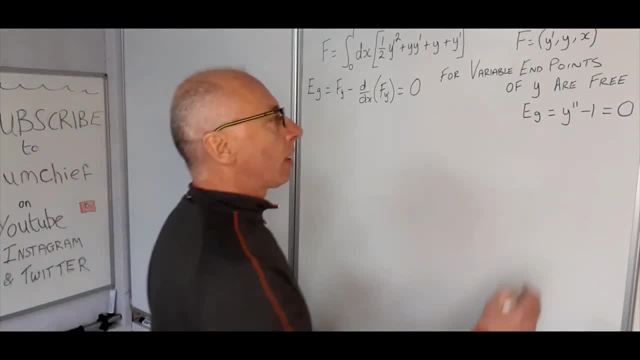 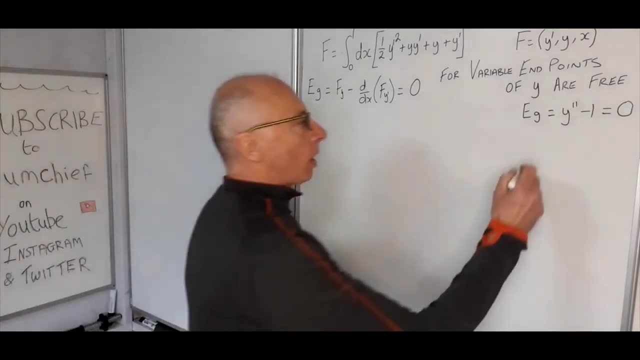 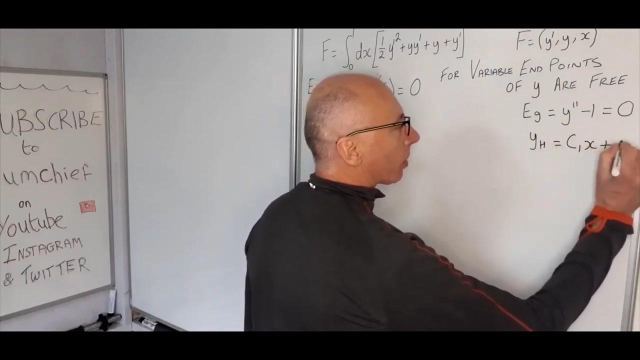 what we need to do now is find the homogeneous solution of this. So y prime minus 1 equal 0.. Now this is a second-order differential equation, so our homogeneous solution of this will be in the form of c1 x plus c2.. Okay, so now. 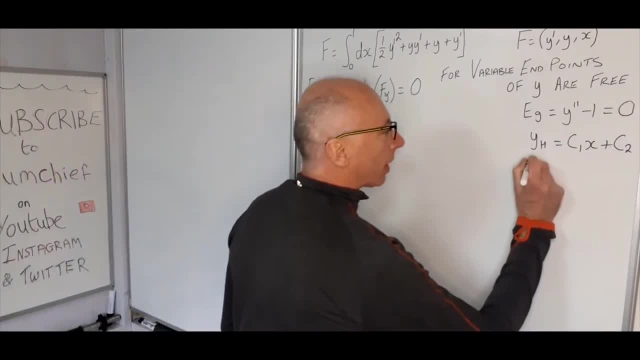 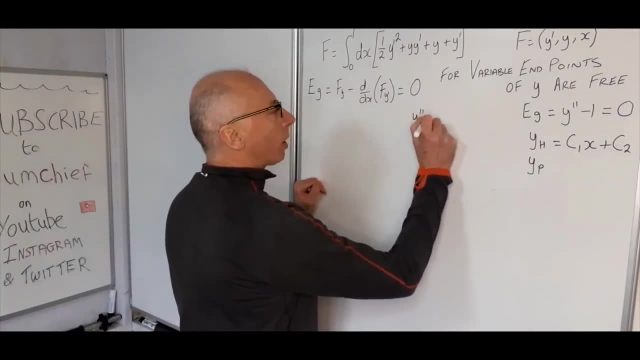 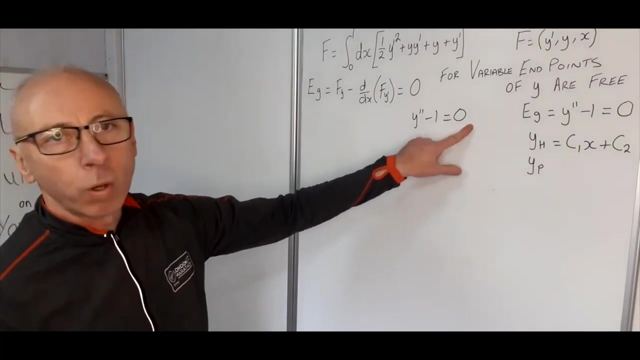 we need to find a particular solution. So let's write that down as a y p. So let's bring this up to here. so y double prime minus one equals zero. now for a particular solution. we don't want a zero in here, so what we can do is we've been the one across. 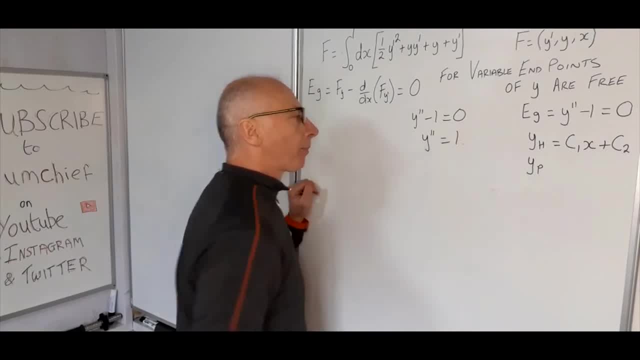 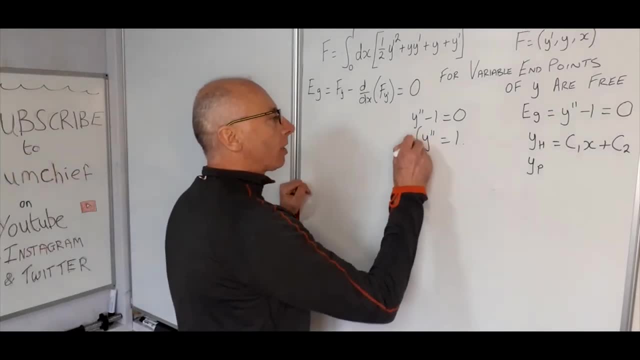 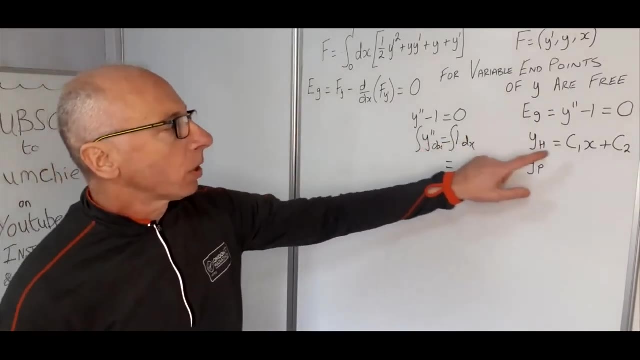 so now we're left with y double prime equals one. okay, now we can take, just integrate twice, and then we can see what happens. so, regards to x, integral, regards to x, now we don't need the constant multiples in here, because we're going to be dealing with them. 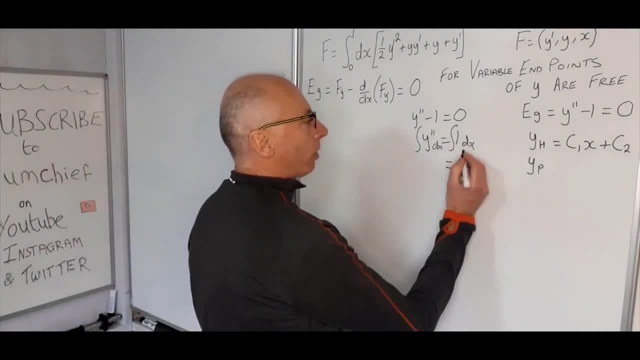 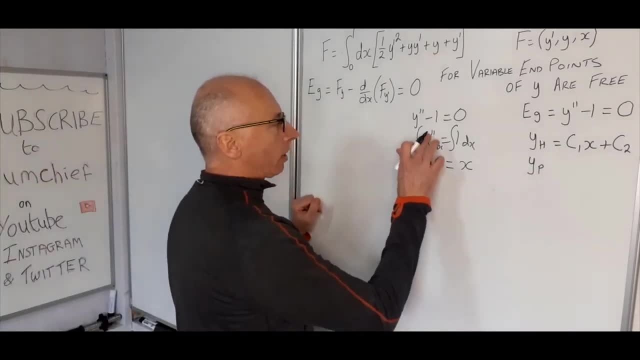 with our homogeneous solution anyway, so the integral of one with regards to x, that just gives us x. don't worry about the plus c. so then let's just integrate this side. we're going to have to be y prime, and then, if we integrate again with regards to x, 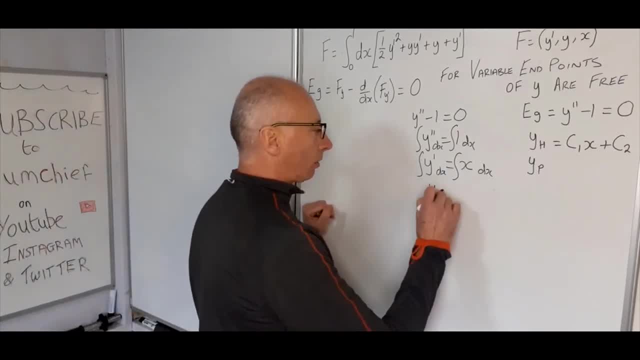 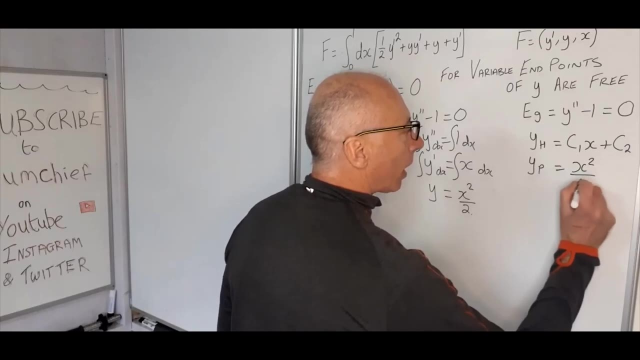 so this will then give us our y that we want. and then, if we integrate again with regards to x, and then if we integrate again with regards to x, then the integral of x with regards to x, simple power rule is just x squared over two. so that's now our particular solution, so that equals x squared. 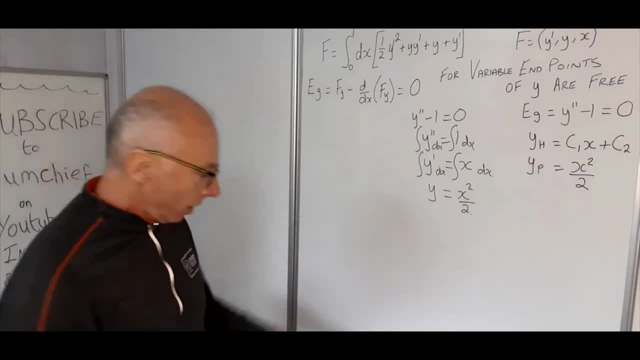 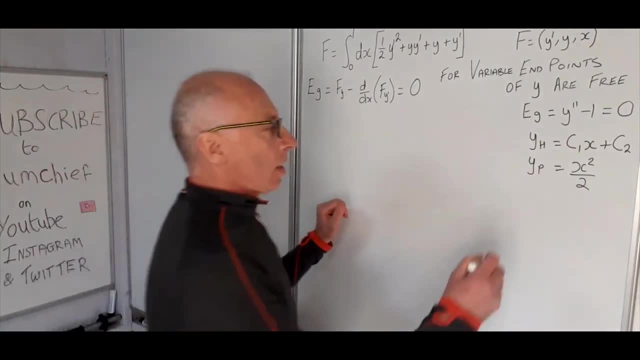 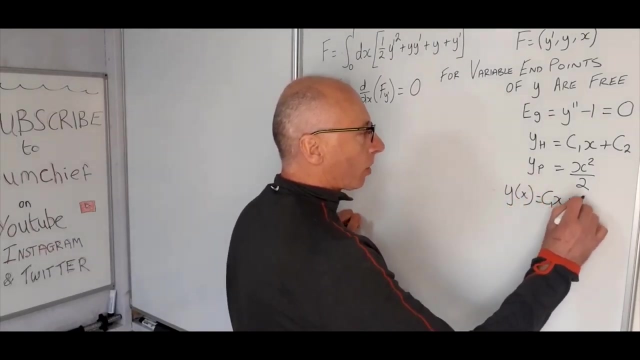 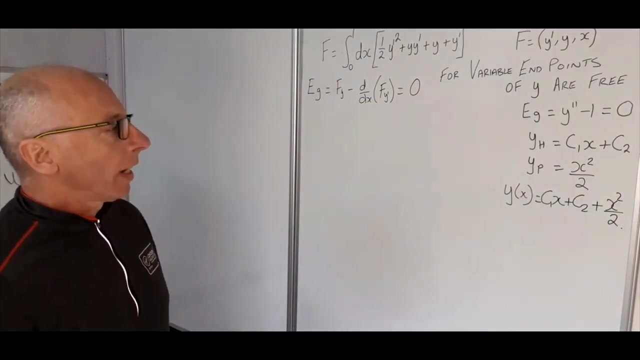 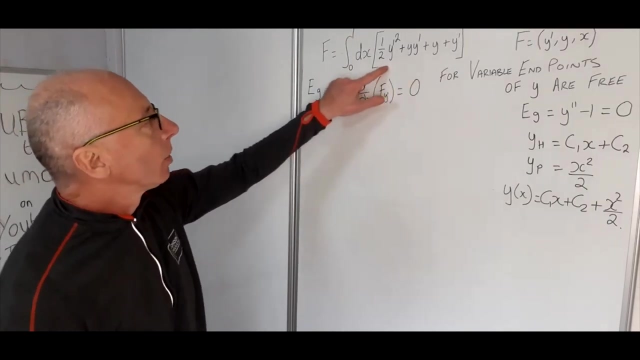 over two. okay, now i'm going to take this off the board. okay, so we've got our homogeneous and we've got our particular. so now what we've got? we've got y of x equals c1, x plus c2 plus x squared over two. okay, so now we're ready to put in our values at x equals 0 and x equals 1 of our partial derivative. 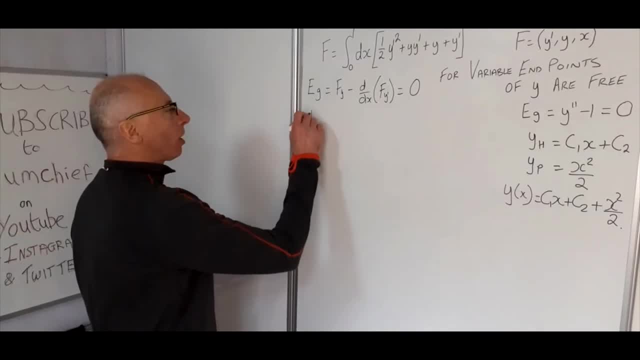 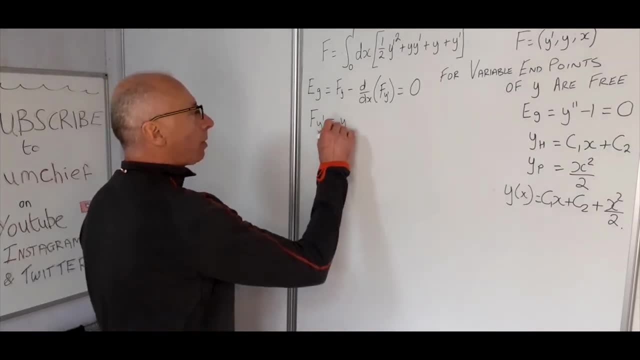 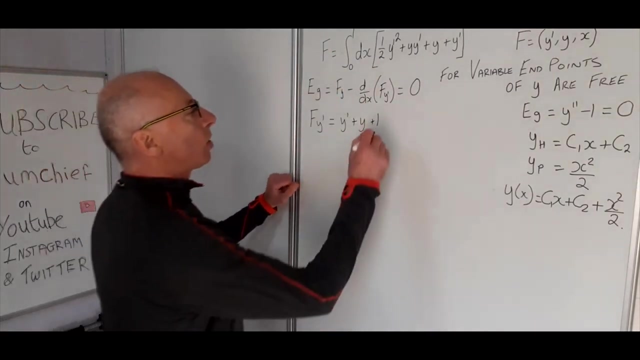 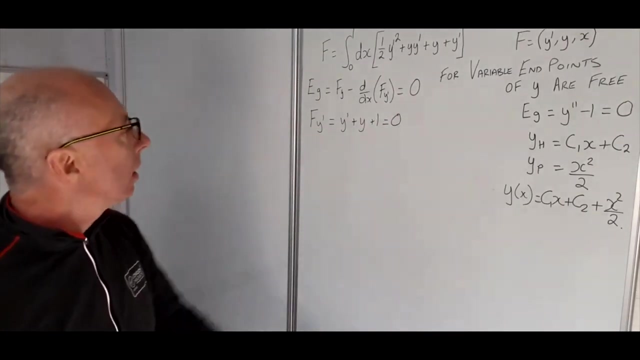 with regards to y prime, which what we previously got was f of y prime. now that equaled y prime plus y plus 1, and we want to know when that's stationary, so that's when that equals 0.. okay, now we've got a y of x here, so now we need to find our derivative of this. 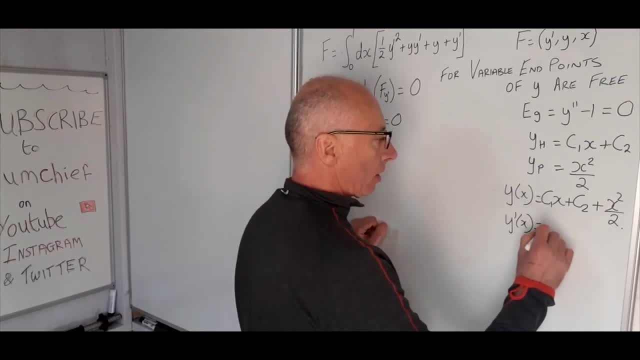 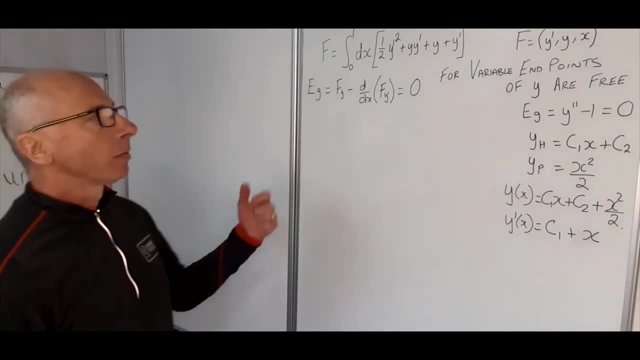 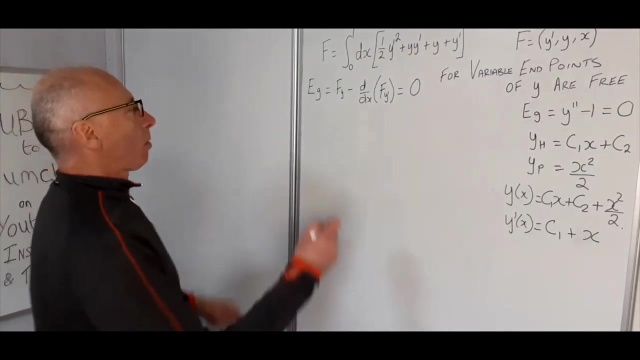 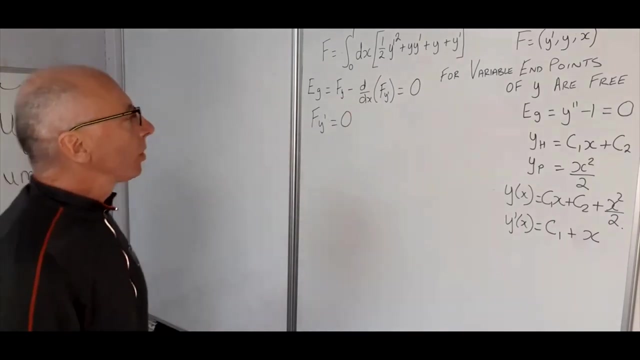 so y prime of x is c1. squared over 2 is just x. okay, now, as this is a variable endpoint problem, what we're interested in is when this f equals x, is when this f equals x, is when this f equals 1.. functional is stationary, so what we want is f y prime when this is equal to zero. now we're given. 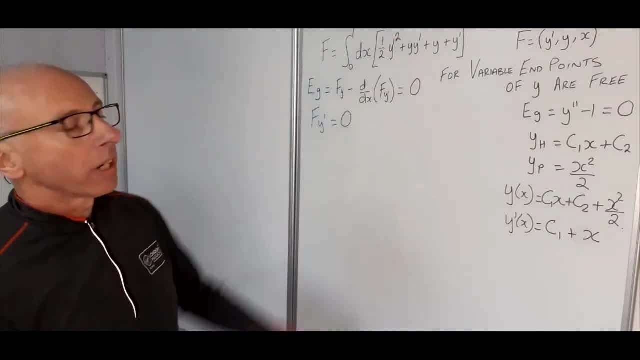 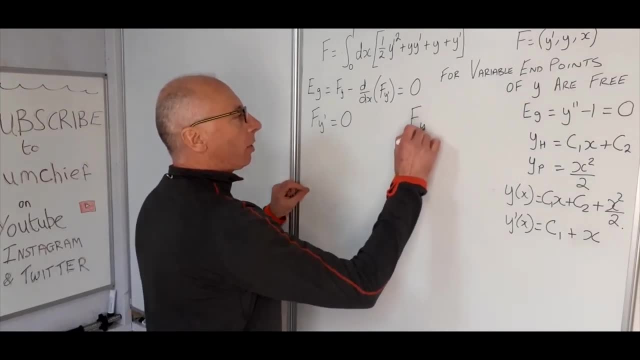 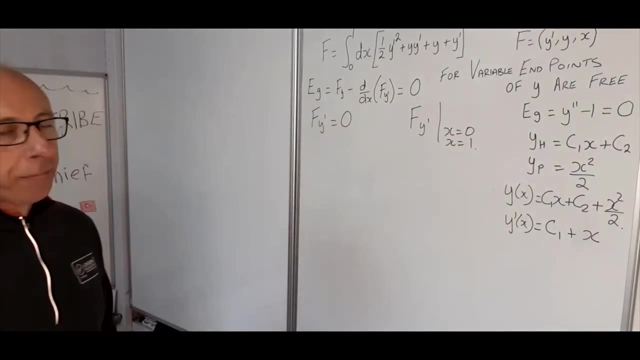 that x equals zero and x equals one is our range of integration. so they're the points that we're interested in. so what we're looking for is f. the partial of f equals to y prime at the points where x equals zero and x equals one. so what we can do is plug in our values at these points for our 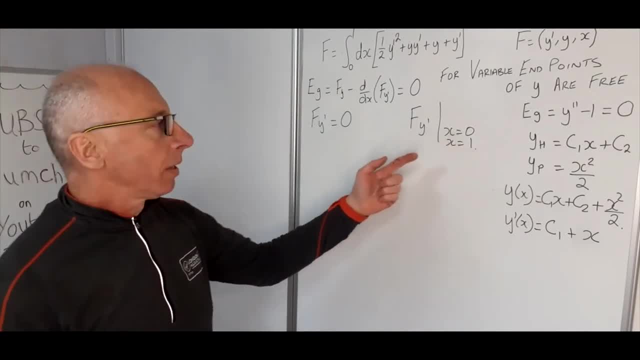 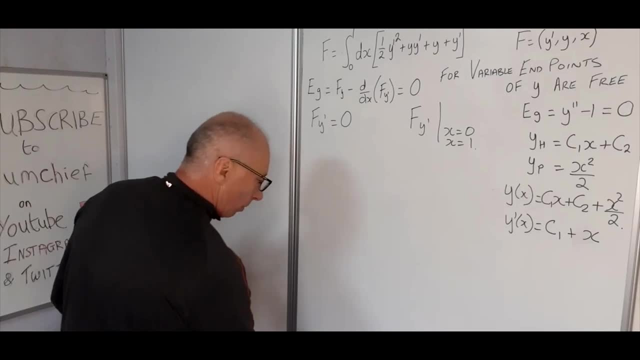 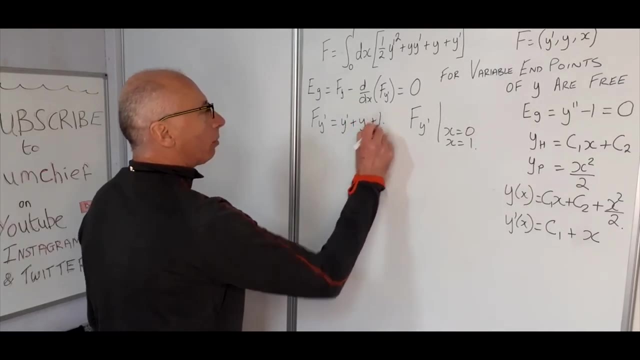 partial of f and see what we can come up with when we plug in the values of x equals 0 and x equals 1.. so previously worked out that f- partial of f with regards to y prime, that was y prime plus y plus one. so now, 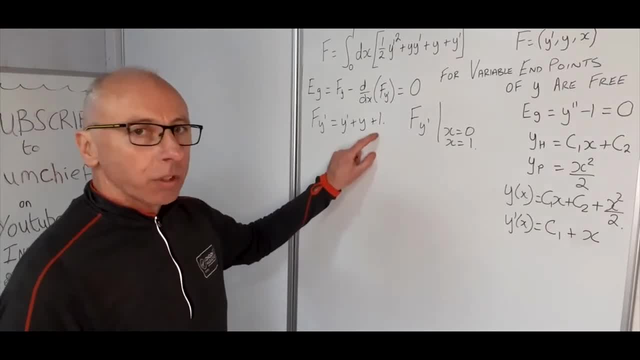 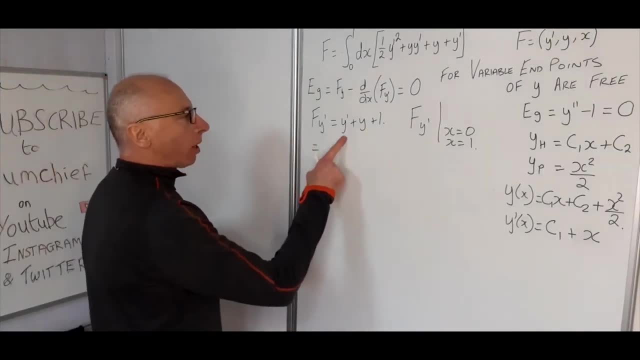 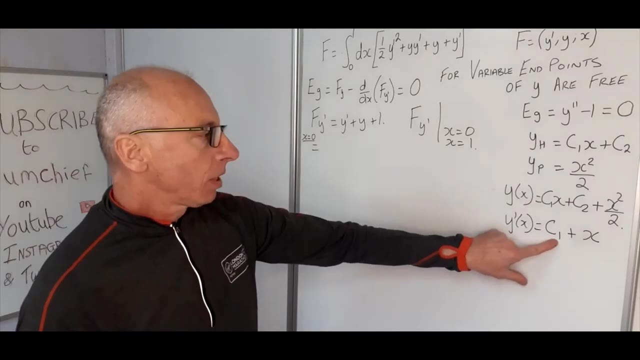 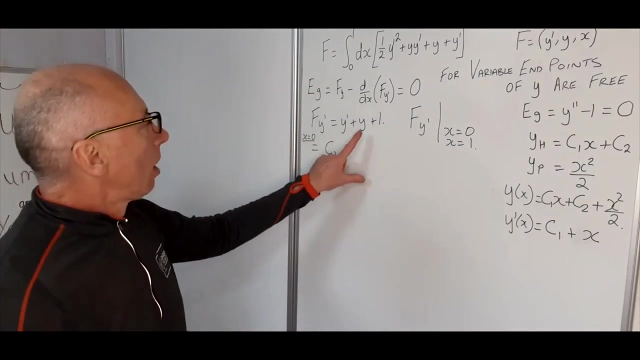 what we need to do is just plug in the values for these functions here at x equals zero and x equals one and see if we can come up with something. so y prime at x equals zero, so x equals zero. let's do that first. so y prime c one plus zero just leaves us with c one. y at x equals zero. that. 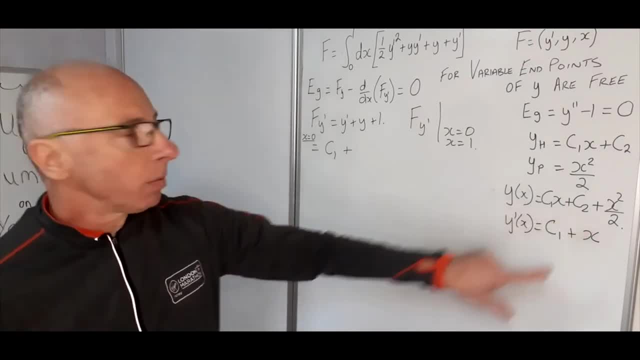 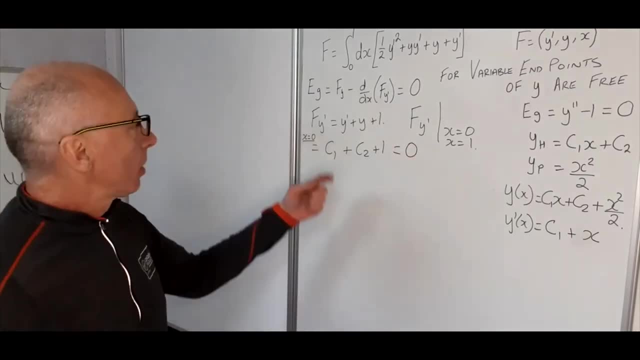 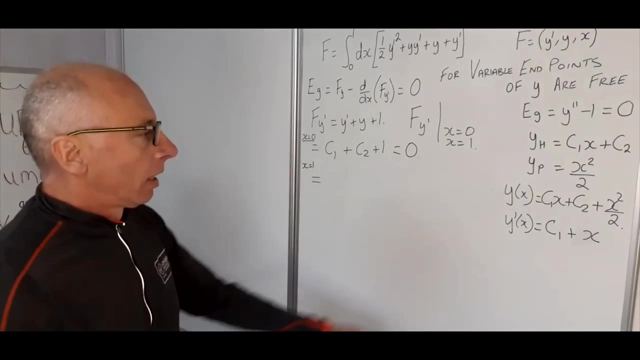 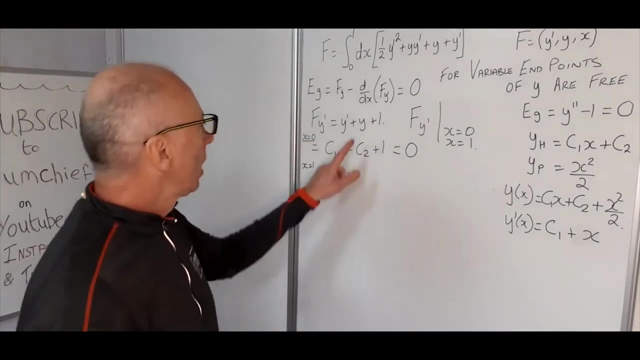 disappears, that will disappear and that leaves us with c two and then plus one that equals zero. so that's at x equals zero there. so what about when x equals one? so if x equals one, we've got c one plus one and our y. so if x equals one, we're left with another c one. 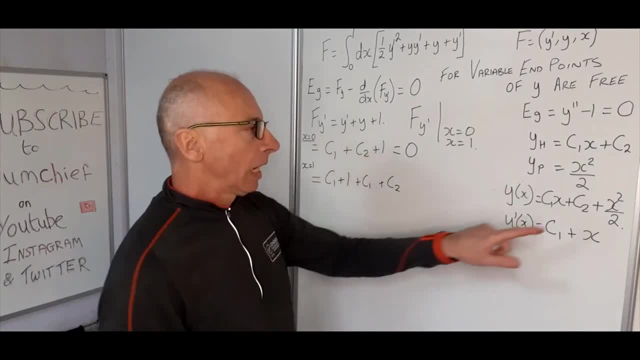 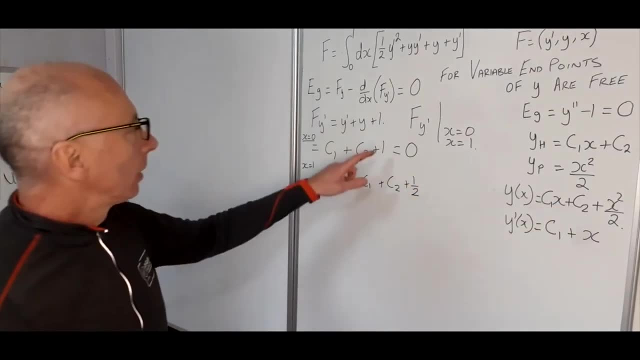 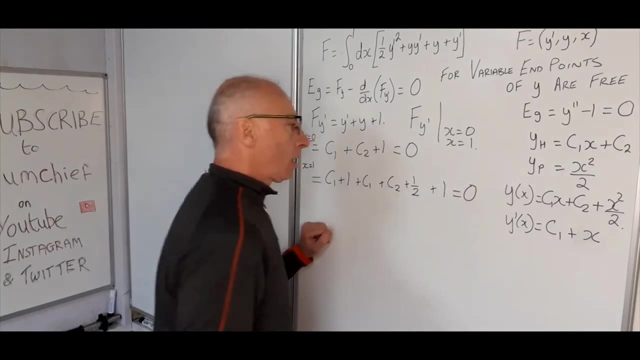 c two again and x equals one here. that's just going to give us a half. and don't forget our 1 here again. so we've got another one and that equals zero. okay, so we can simplify this up a little bit so the c two can stay on its own. that's just a one, but 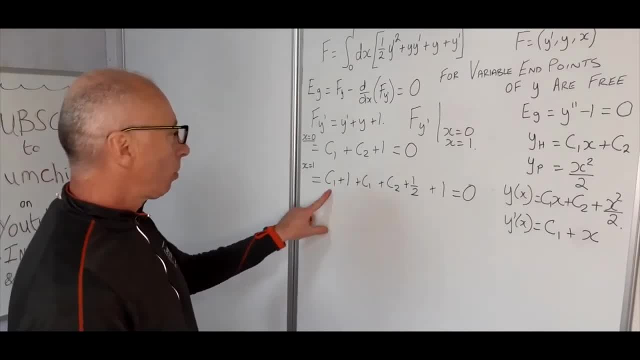 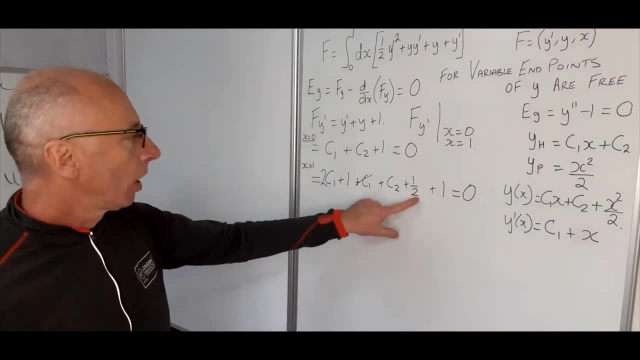 the c one. we've got two of them, so we can cross that one off and put the two there and that's it. so we can simplify that here and that's it and put a 2 there And the constant multiples. we've got a 1, a half and a 1.. 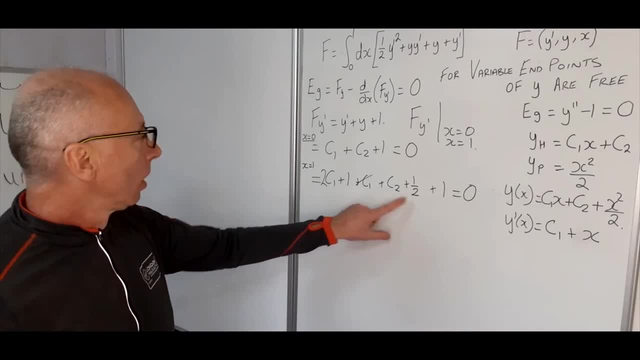 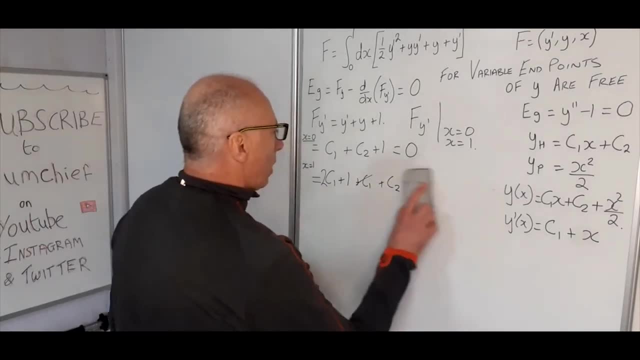 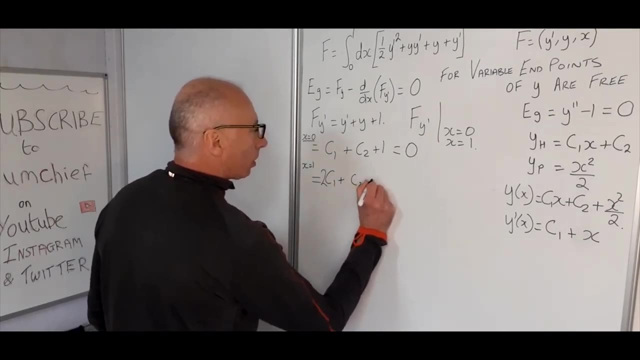 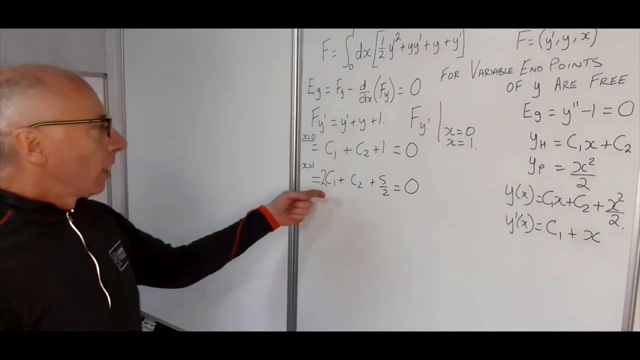 So that's set to 5 over 2.. So 2C1 plus C2 plus 5 over 2 equals 0. So let's just put that in there a little bit. So 2C1 plus C2 plus 5 over 2 equals 0.. Okay, now we're. 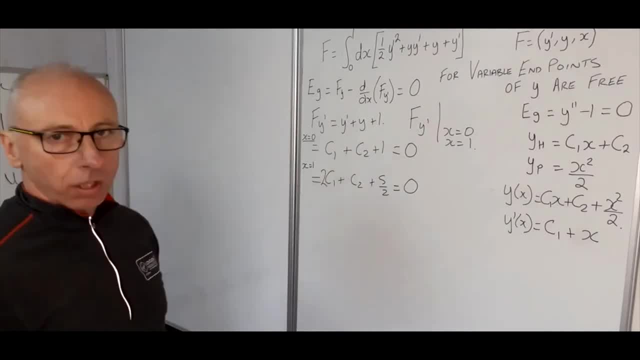 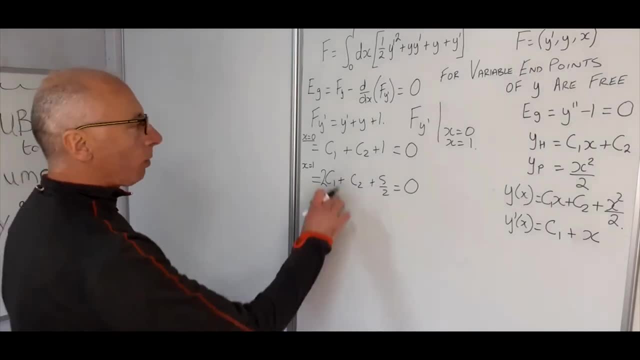 interested in our arbitrary constants C1 and C2.. Now we've got looks like here: we've got ourselves a good old fashioned simultaneous equation. So if we subtract this one from this one or vice versa, we can get rid of the two. So we've got a 2C1 plus C2 plus 5. 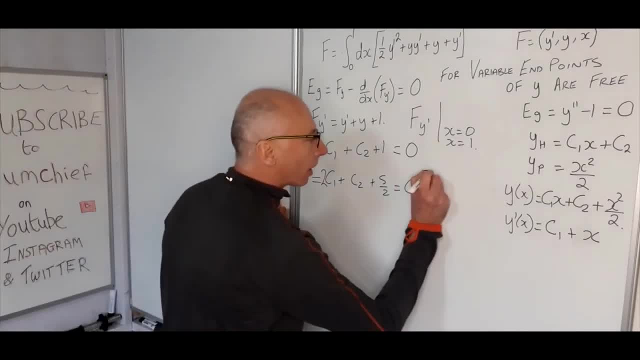 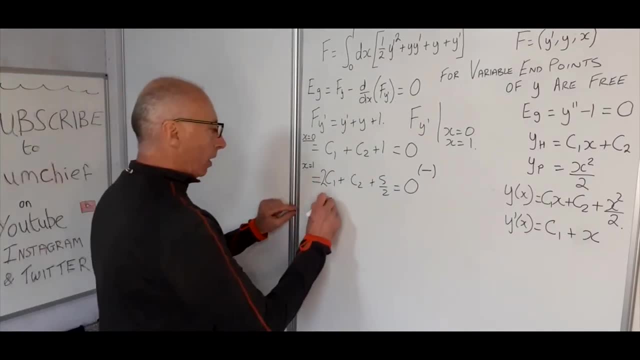 the c2. so if i put a minus sign here as our action we're going to perform on these two, c1 minus 2, c1 that gives us minus c1, c2 minus c2, that disappears, and then 1 minus 5 over 2. 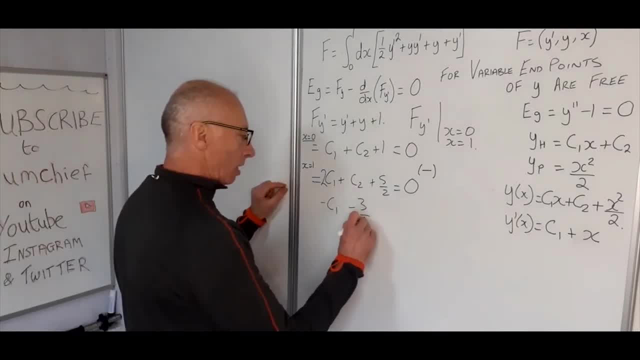 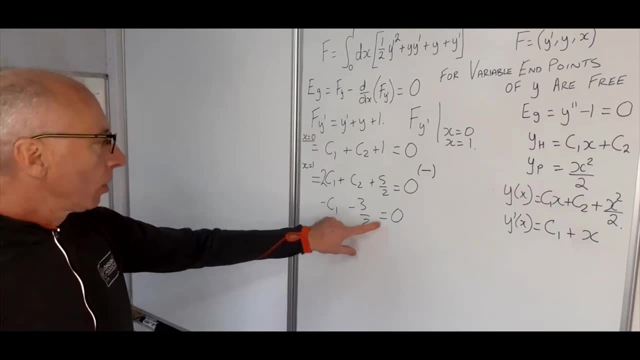 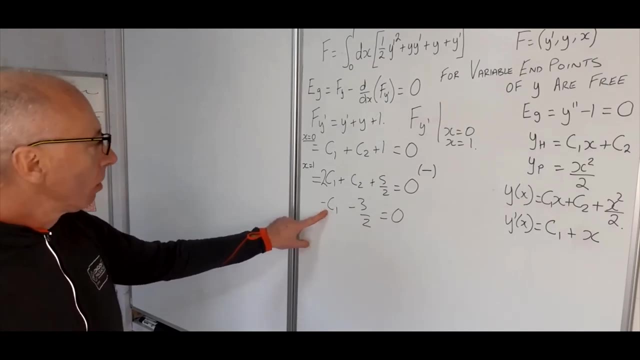 gives us minus 3 over 2 and that equals zero. so what does c1 have to be for? minus 3 over 2 equals 0. well, if c1 is minus 3 over 2, 2 minuses, make a plus 3 over 2. minus 3 over 2 equals 0, so we can.